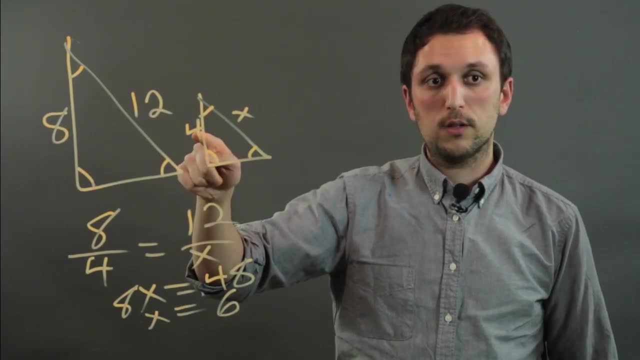 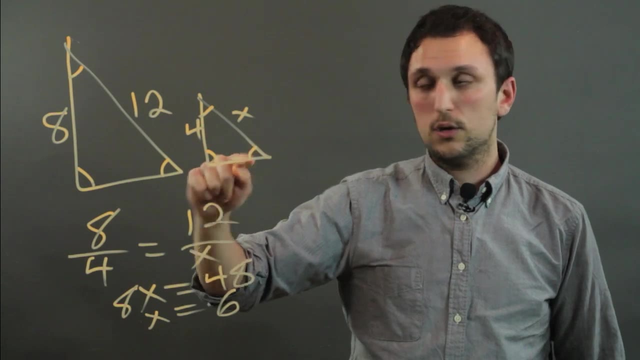 use a similar triangle. most often times You have one leg that corresponds to another. thus any other leg corresponds to any other, proportionally. So the hypotenuse and the hypotenuse. if this were a right triangle, or the a-leg and the a-leg and the b-leg. 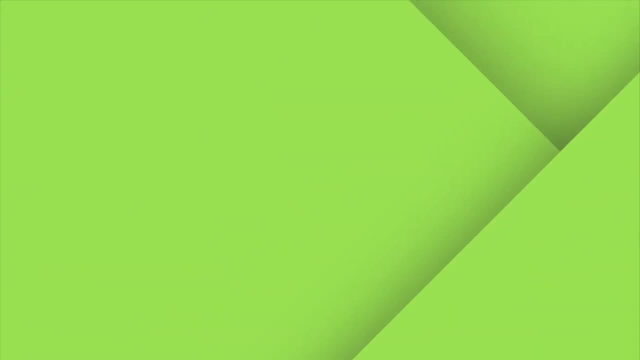 and the b-leg. Thanks a lot. Subtitles by the Amaraorg community. 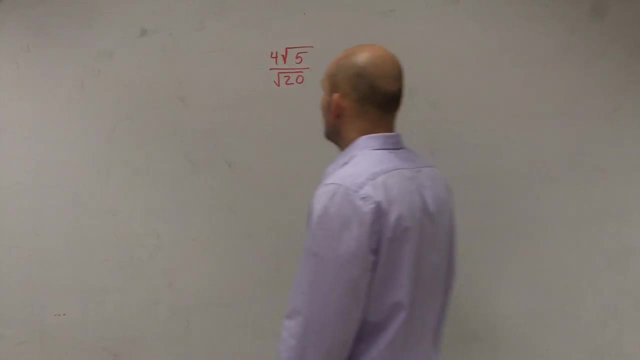 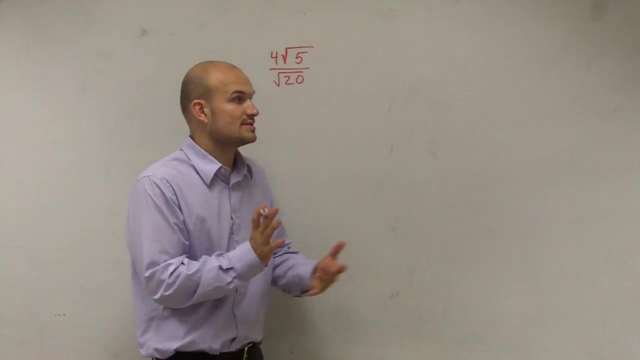 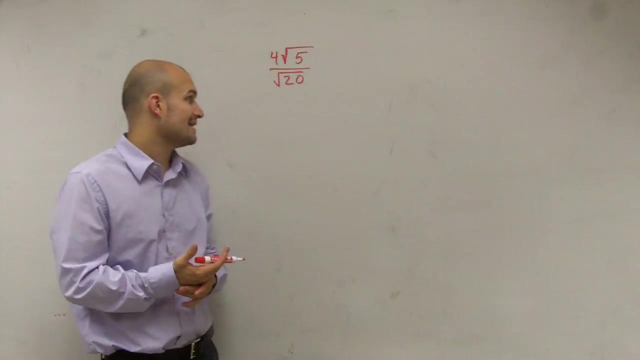 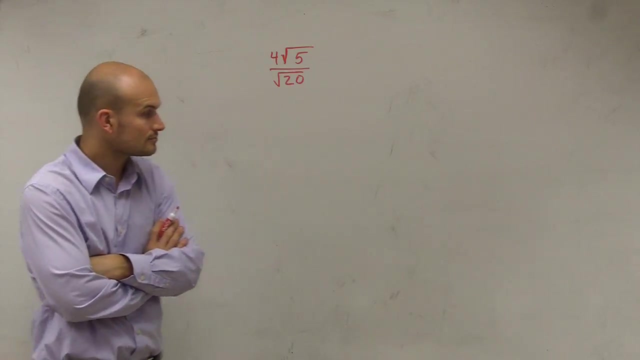 So, ladies and gentlemen, if I want to simplify this, the main important thing is: we've talked about adding and subtracting, alright, and when you add and subtract, you've got to have them in like terms. Well, the same thing, when we're multiplying, we can multiply across. However, we have a problem here. If we're going to be dividing, alright, when we're dividing, one thing is: you know, we can't divide into by our radical. So what I'm going to want to do is I want to see, can I simplify either the square root of 5 or the square root of 20?? 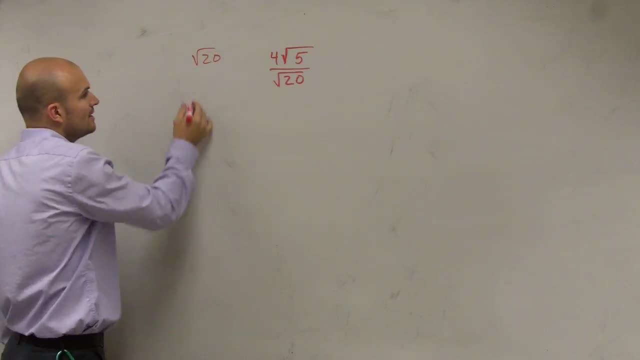 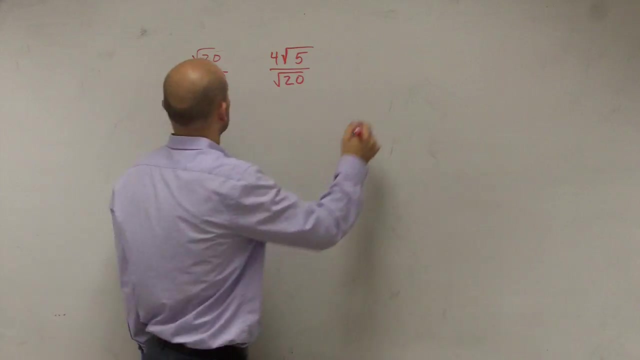 And let's kind of go off to the side. Well, I can simplify the square root of 20.. I can rewrite that as square root of 4 times 5, right Now. some of you might say, well, yeah, that's pretty good, but you can also do square root of 20 as the square root of 10 times 2, right, Right Now. why do we want to do it this way rather than that way? Does anybody want to raise their hand and tell me that one? 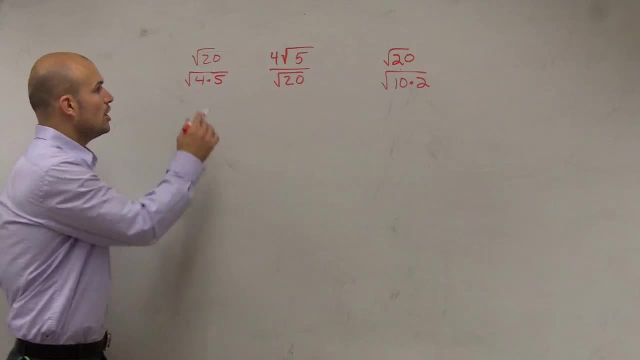 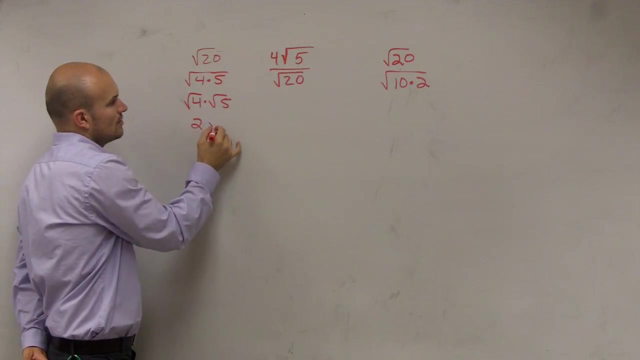 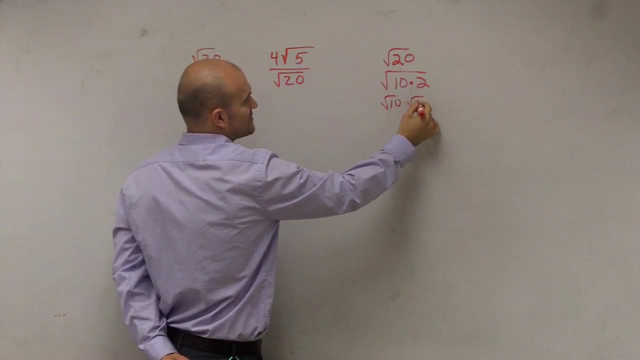 Yes, exactly because 4 is a square number. We know what the square root of 4 is. The square root of 4 is 2, right, So I get 2 radical 5.. But, ladies and gentlemen over here, do you know what the square root of 10 is, or the square root of 2?? 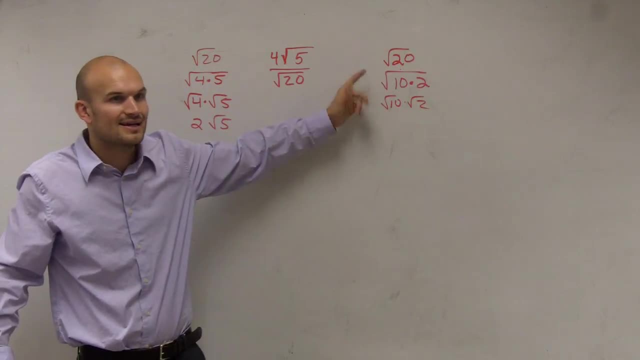 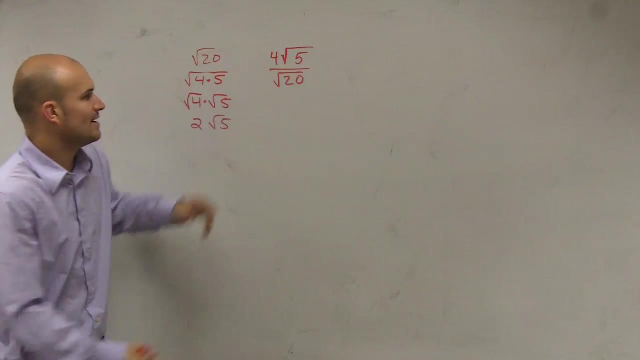 No. So even though this is mathematically fine, it's not going to help us simplify it. So what I do is now I can rewrite this as 4 radical 5 divided by- oh, I'm sorry, not radical 2.. 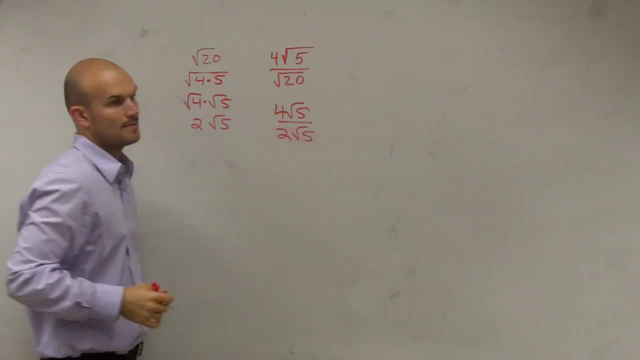 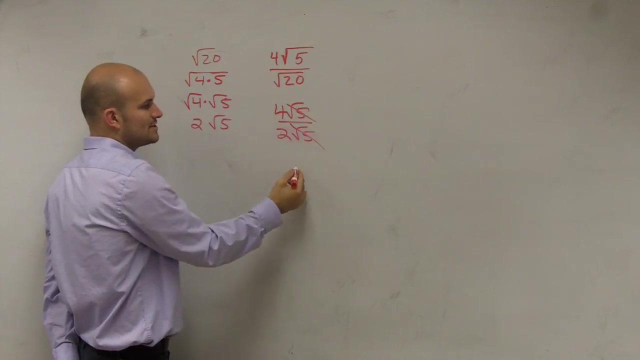 It's 20, but 2 radical 5.. And then what you guys will notice, Stephen, is that the radical 5s cancel out and you get 4 divided by 2, which just equals 2. And there you go, That's it.